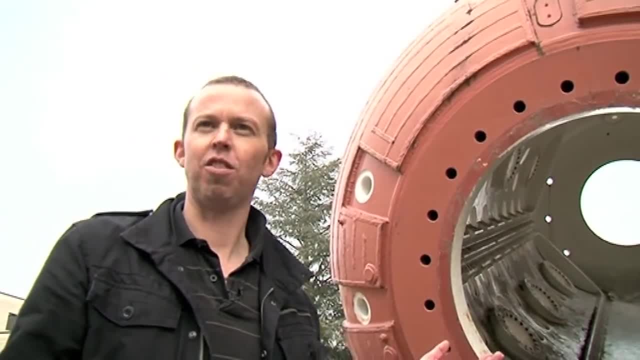 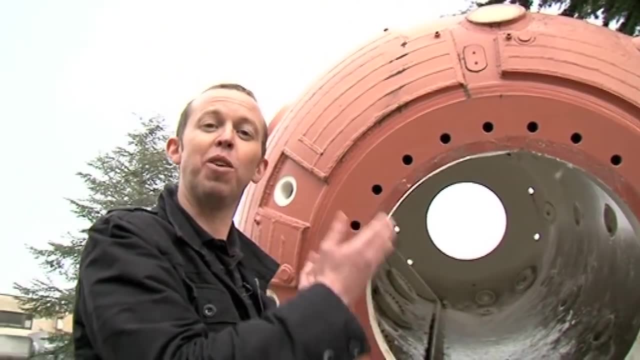 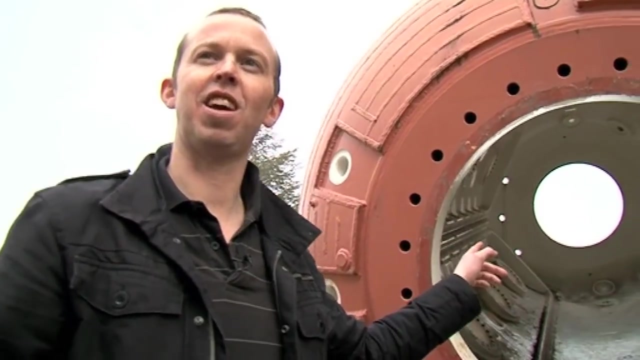 However, if you've got a neutral particle passing, an electron, something with no electromagnetic charge, you wouldn't expect anything to happen, Except when there's another interaction involved, And that other interaction is called the weak interaction, And that's what was measured inside this chamber back in 1973.. 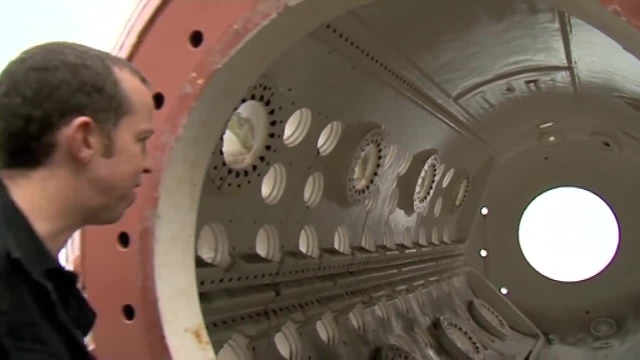 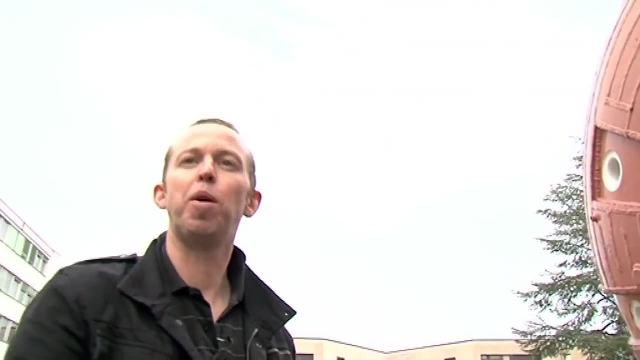 So this is a piece of history, is it? It really is a piece of history. The experiment that went on in this machine actually won Glashow, Weinberg and Salam the Nobel Prize in 1979. What happened in this? They've got a lot to thank this machine for. 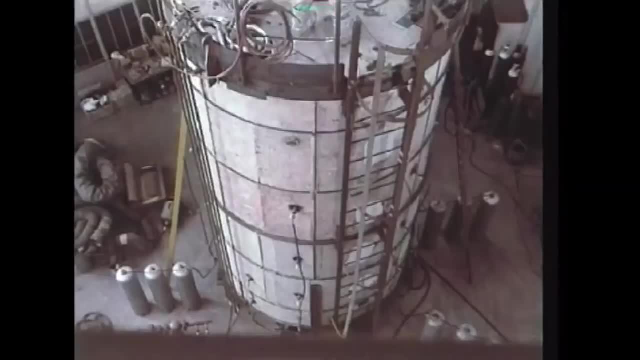 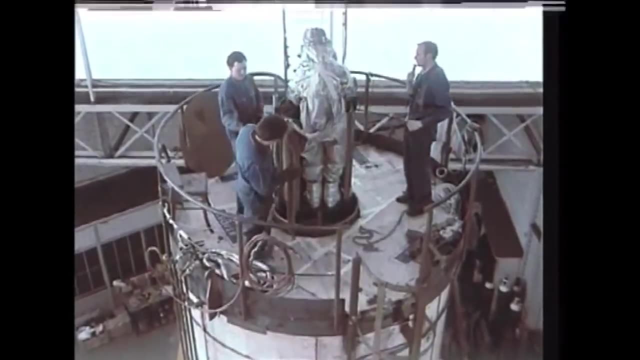 The body of Gargamel's chamber is a huge can container, 4 meters 80 long and 1 meter 90 in diameter. It's got two holes. The construction required a far greater precision than that needed in conventional boiler making. So we're in the science garden in CERN where there's a lot of little bits and bobs of equipment. 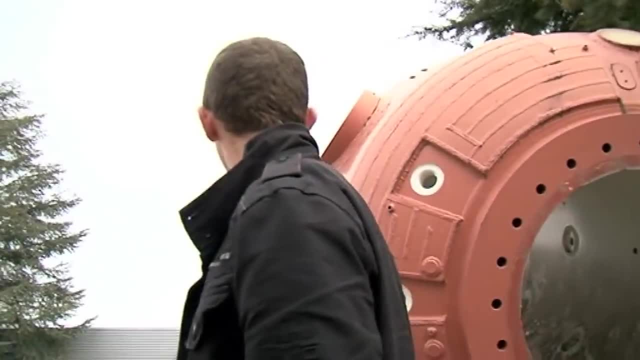 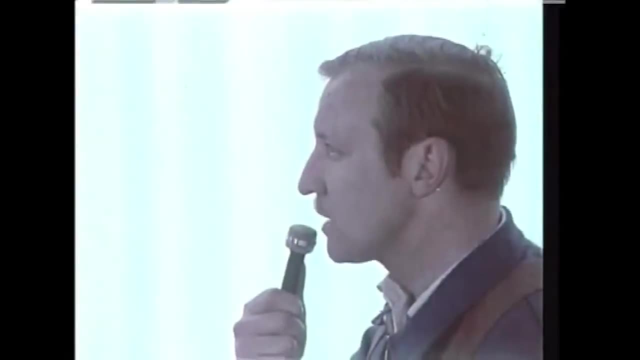 Some of it's just been put together as art. This is obviously its original thing. This used to weigh 25 tons when it was full of Freon. To guarantee good photographs, the inside of the chamber has to be painted with an absolute photographic black. 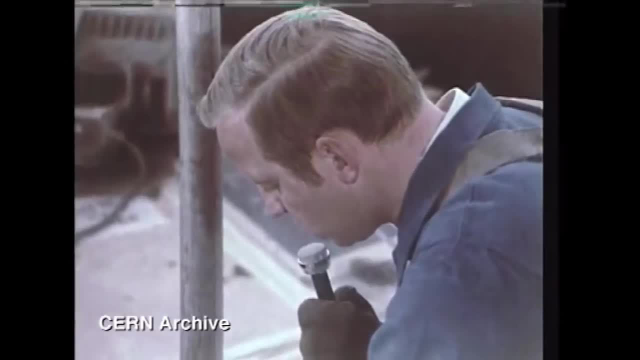 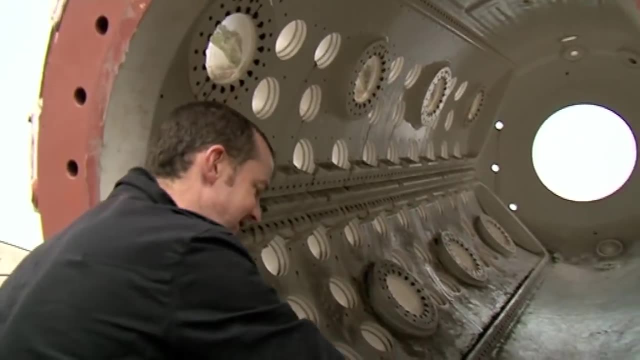 against which the thin, slender strings of white bubbles stand out clearly. It's in a terrible state. This is disgraceful. There's like a beer can, right? I don't know if this was Weinberg came along here to celebrate or what, but this is a. 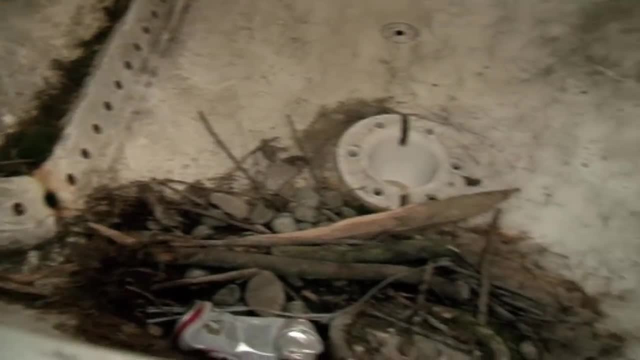 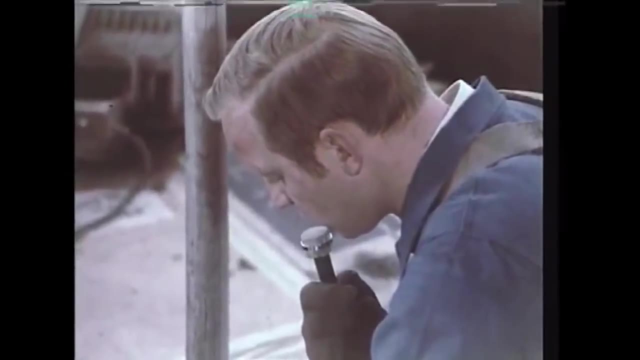 Oh, I don't even want to touch that. There's a cigarette butt down there as well, It seems to. It's a bit disappointing, really, that they let it get to this state, when this is really scientific history. An epoxy resin paint was used. 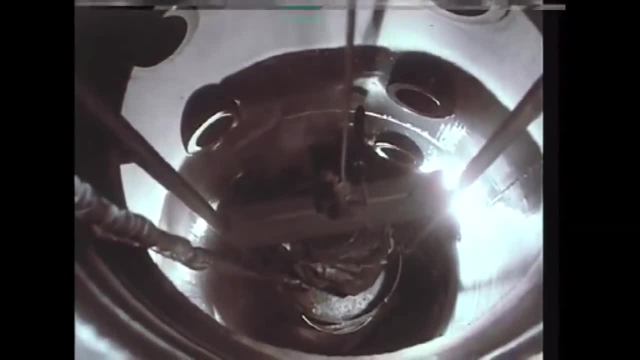 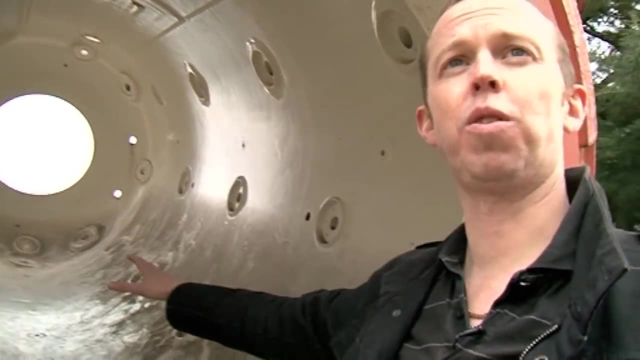 It was applied by an operator wearing a special heatproof suit, for he was working in a chamber heated to 120 degrees At the time of the experiment back in 73,. this was full of liquid Freon And then they passed some neutrinos through it and there were some electrons knocking around. 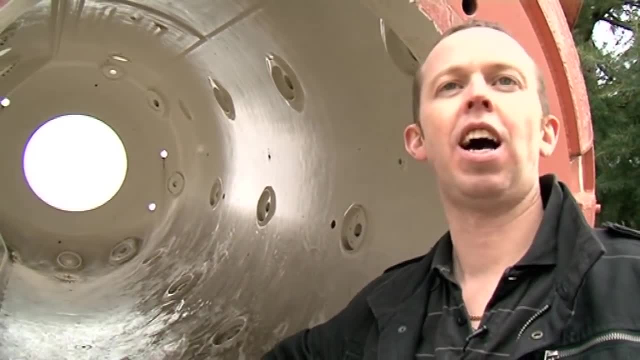 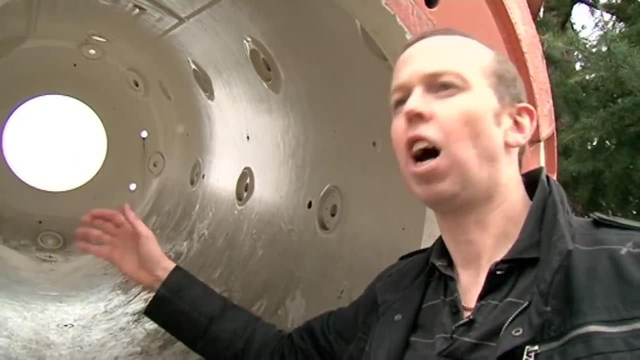 Now, if you just had the usual electromagnetic interaction, nothing would happen. That neutrino's got zero charge. It's not going to do anything to that electron. Okay, there'll be a gravitational attraction between the two, but that's tiny. 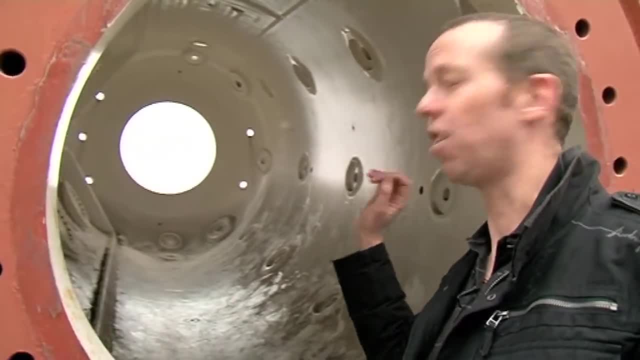 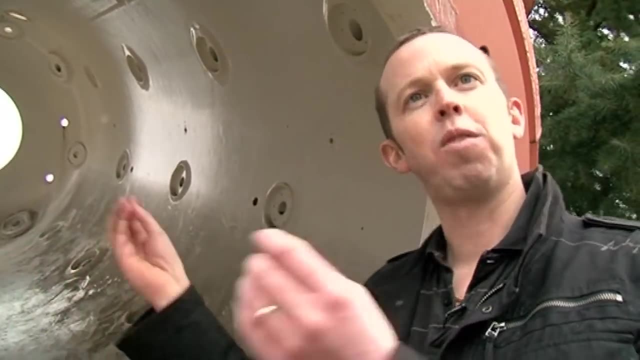 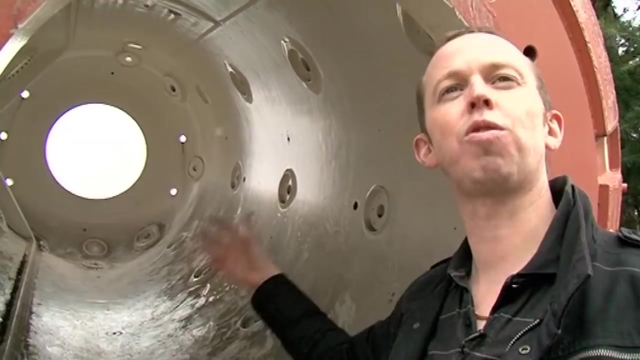 You're not going to observe that, So you wouldn't expect anything to happen, except Weinberg and Glashoff and Salam predicted that something would happen, that there would be this neutral current between them, that basically this neutrino and this electron would exchange what's called a Z particle. 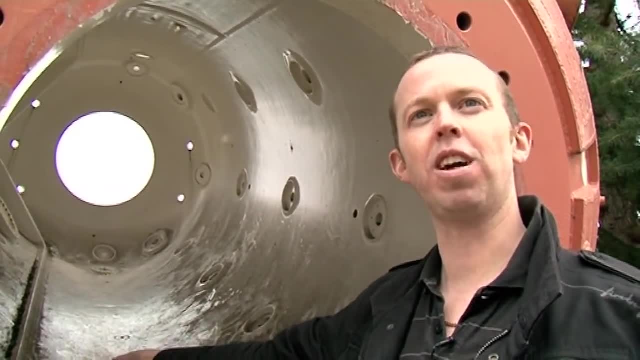 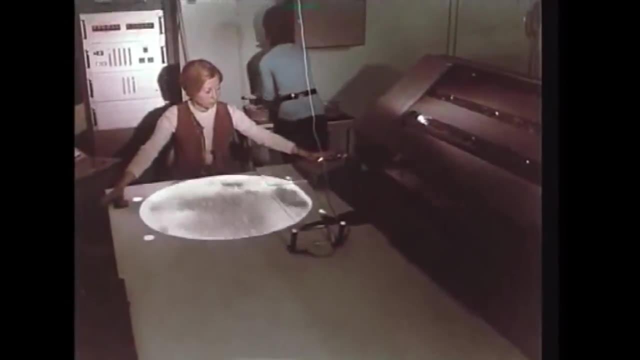 Okay. so that Z particle would go between the two objects and it would cause the electron to sort of judder a little bit, to wiggle around a little bit, And that happened. That was seen in here. Basically, they threw loads of neutrinos through this thing to make sure it happened. 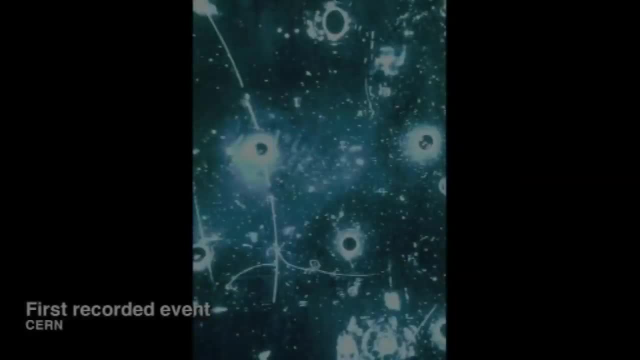 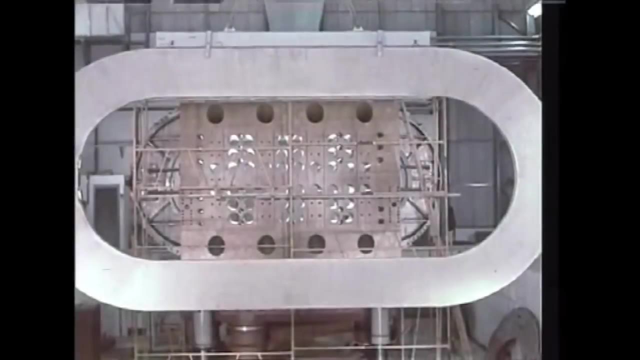 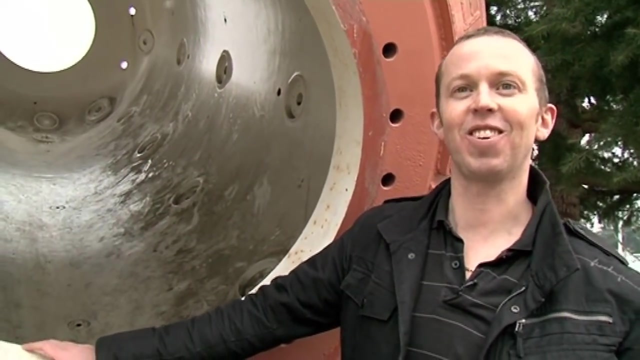 And the electrons started to wiggle And that was proof that, because we knew there was no electromagnetic interaction. that was proof of a new type of interaction taking place inside this machine. It's the weak interaction. It happens in the sun. Okay, it's what makes the sun glow. 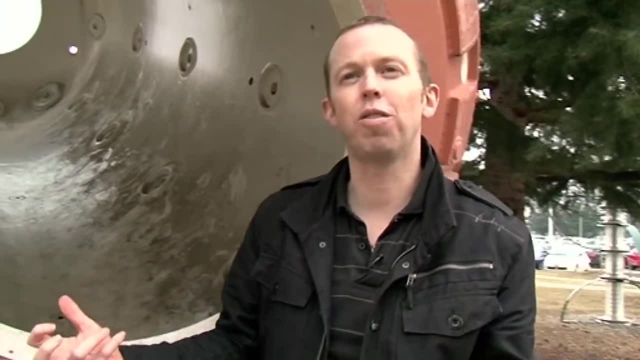 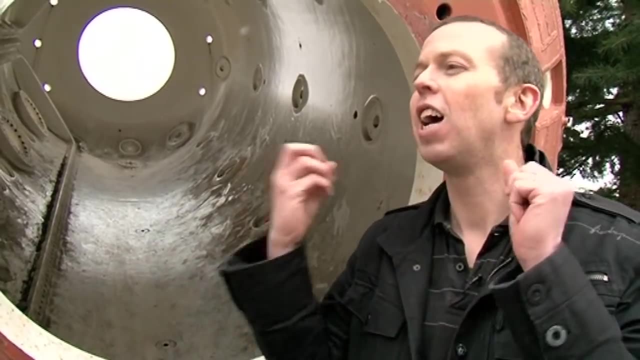 So you know what happens in the sun, for example, is a neutron will decay into a proton, an electron and a neutrino. That decay process happens in the core of the sun. It's essentially what makes the sun glow. 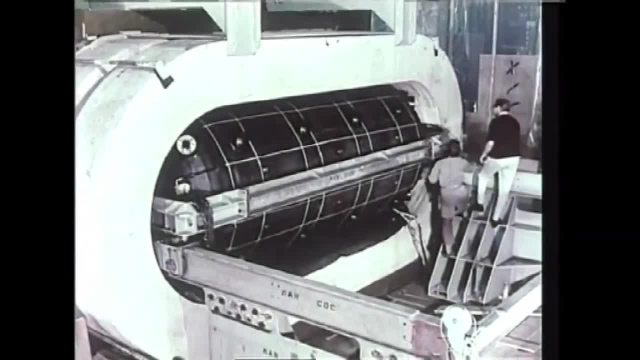 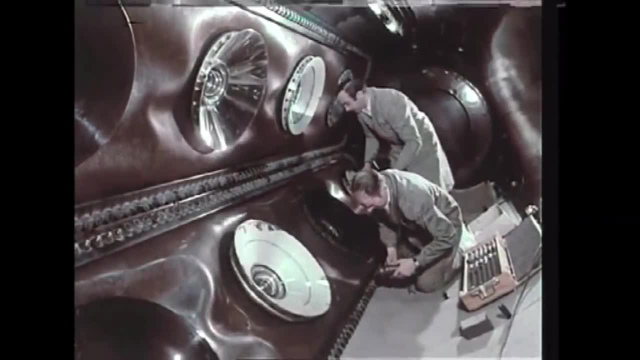 That process is essentially due to the weak interaction. It's a weak process In front. there is enough room to allow the chamber body to be set up. What Weinberg, Glashoff and Salam did? they merged electromagnetism and the weak interaction together. 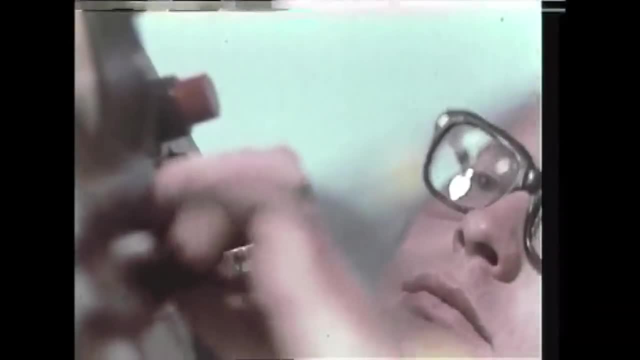 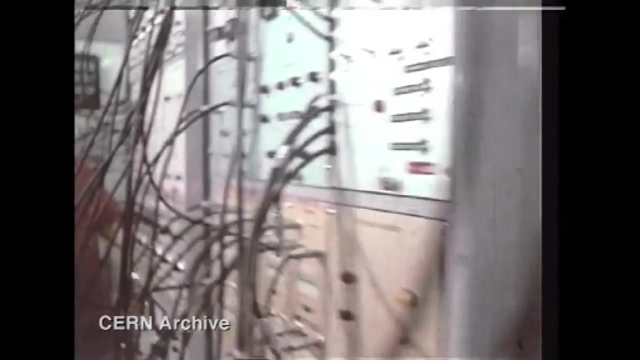 in a unified theory called electro-weak theory. Gargamel costs 25 million francs or close to 5 million dollars. So gargamel is the mother of gargantua in Rabelais' 16th century books on giants. 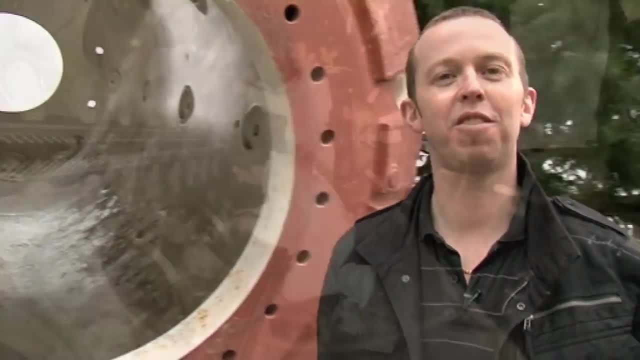 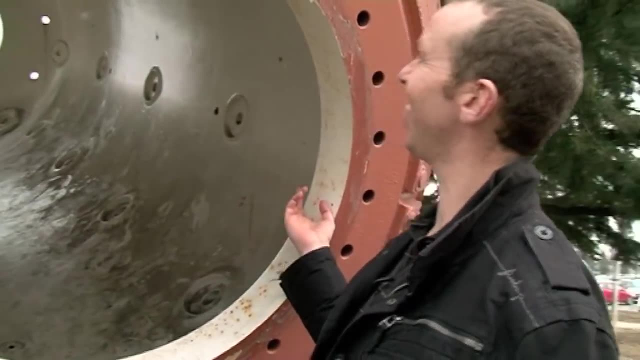 So it is pretty big. It certainly weighed a lot- It was 25 tons at the time of the experiment, so a pretty big object. I did say it didn't look as big as I thought it was going to be, but it doesn't look like 25 tons. 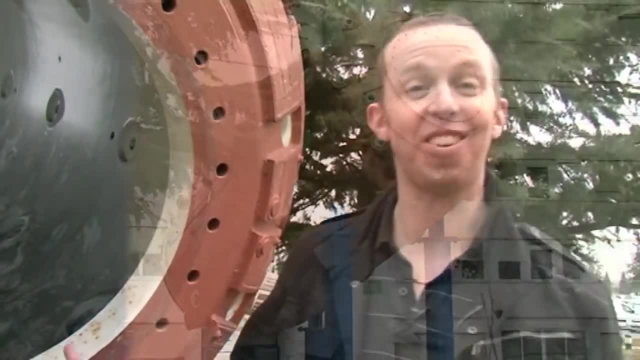 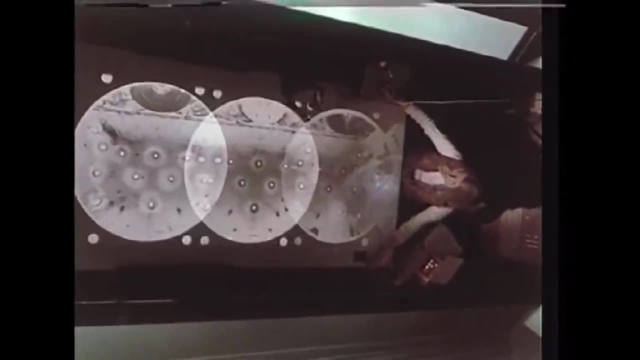 It is a bit underwhelming when you actually see it, but scientifically it's definitely a giant what happened in here. But for the selection of the photographs, nothing can quite replace the eyes of the scanning girl in the hunt for the tracks of the whimsical neutrino.